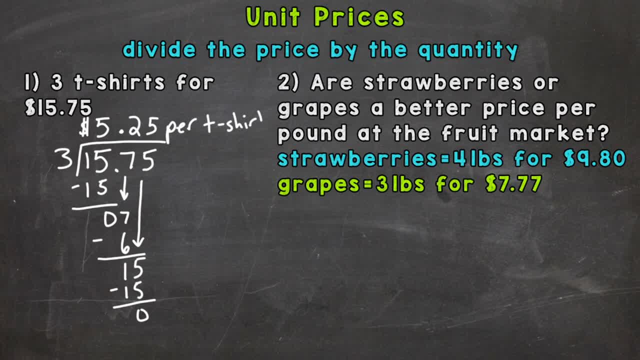 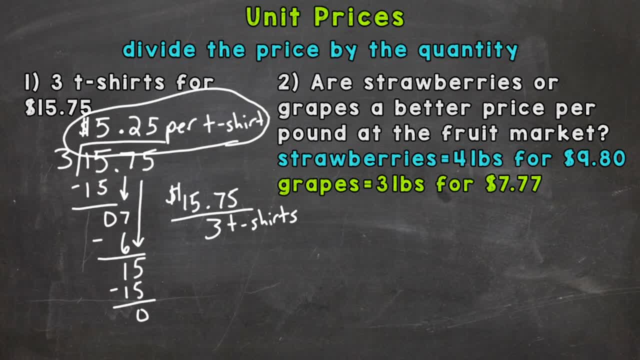 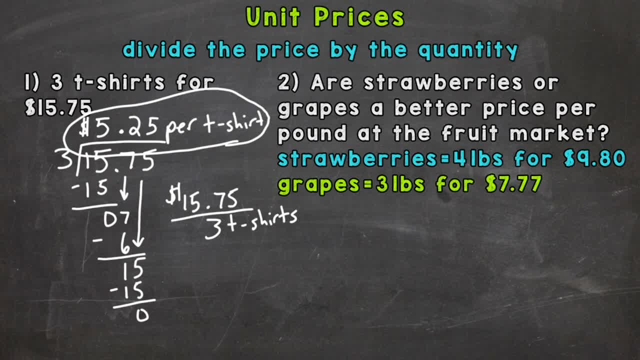 take a look at number two. Are strawberries or grapes a better price per pound at the fruit market? Strawberries are four pounds for nine dollars and eighty cents. Grapes are three pounds for seven dollars and seventy seven cents. So we need to find out which one is less per pound. So again, divide. 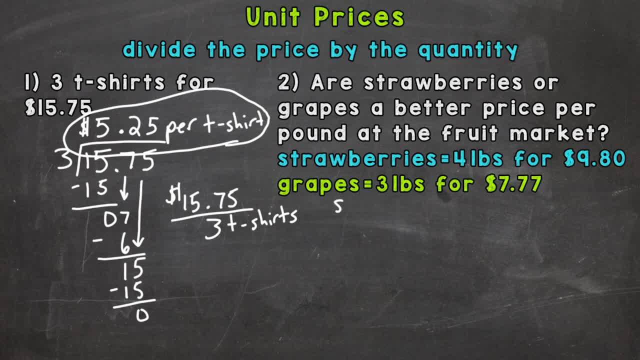 the price by the quantity. So strawberries, So strawberries, nine dollars and eighty cents divided by the quantity of four pounds. So we need to see how much they cost per pound. So we're seven up correctly. Now it's just a matter of solving Nine divided by four. We can pull two whole fours. 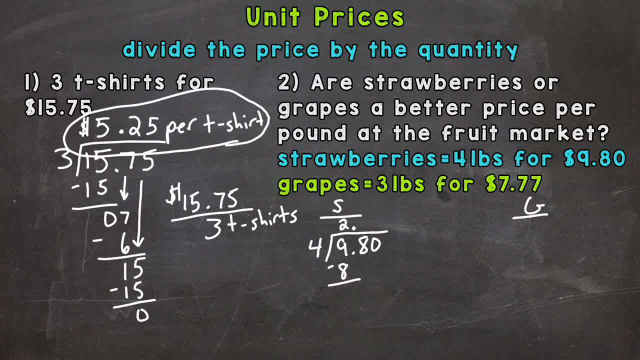 out of nine. Two times four is eight. Subtract We have 18 now And we can pull four whole fours out of 18.. That brings us to 16.. Subtract We get two. Bring down the zero: 20 divided by four is: 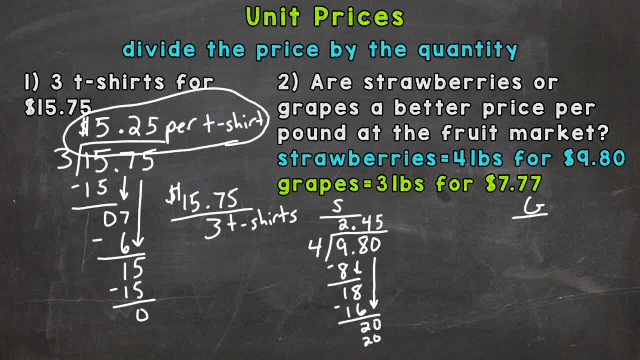 five. Five times four is 20.. Subtract, We get zero. So strawberries are two dollars and forty-five cents per pound. Let's check grapes now. So grapes are seven dollars and seventy-seven cents, and that is for three pounds. So now let's divide Seven. divided by three, We get two. Two times three is six.